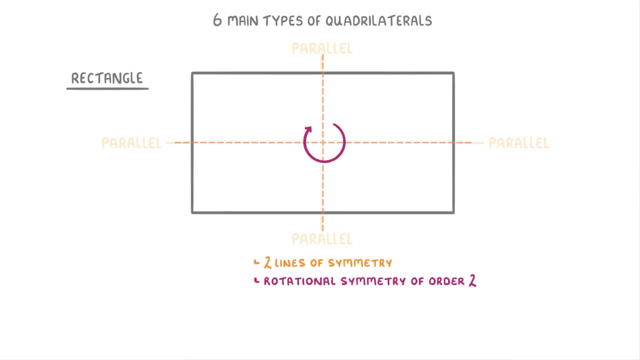 only have two lines of symmetry and rotational symmetry of order. two. Just like squares, though all the angles are 90 degree right angles. Now a rhombus is kind of like a square that's being pushed over. To see what I mean, imagine we had this square and we pushed it up here in the top left corner. 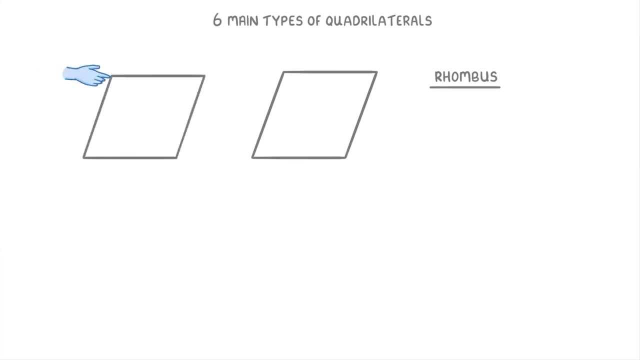 It would sort of lean over to the right, And this shape that we're left with is a rhombus. Also, if we rotate it a little bit, then it ends up looking like a diamond, And in fact you may sometimes hear rhombus being called a diamond, But just remember that rhombus. 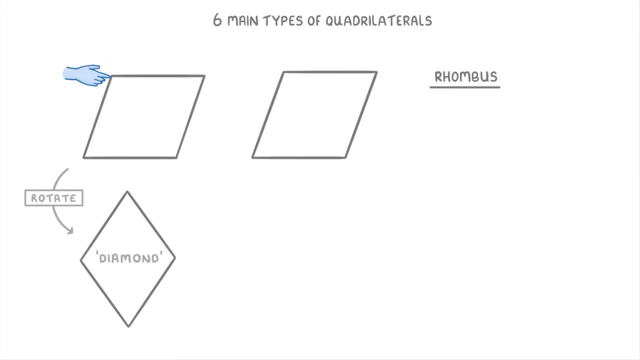 is the proper name for it, But because it came from a square, all four sides of a rhombus are equal length. So instead, but because it's been pushed over, the angles aren't 90 degrees anymore, Instead two of them. 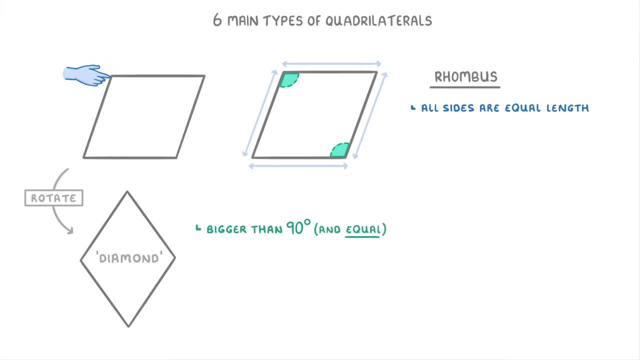 will be bigger than 90 degrees and equal to each other, and the other two will be smaller than 90 degrees and equal to each other. So, in total, rhombuses have two pairs of equal angles. They also have two pairs of parallel sides, so these two sides are parallel and these two sides are 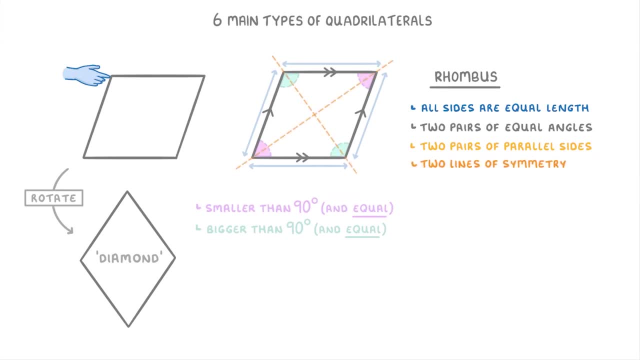 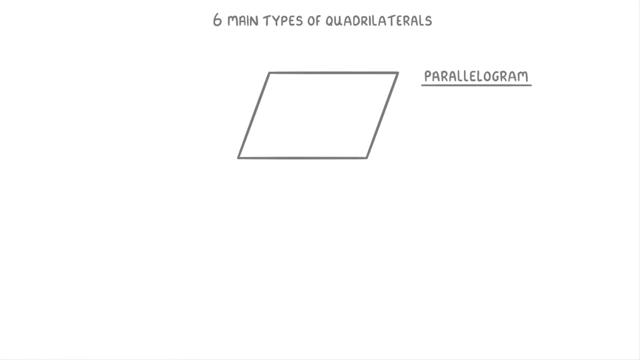 parallel. Lastly, they have two lines of symmetry and rotational symmetry of order 2.. Next up, we have the parallelogram, which is very similar to a rhombus, except it's a pushed over rectangle rather than a pushed over square. So, just like the rhombus, it has two pairs of equal angles. 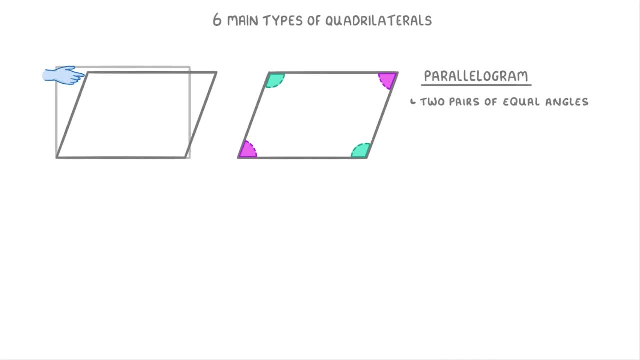 Because it came from a rectangle, though the sides aren't all the same length. Instead, it has two pairs of equal sides, So these two are equal length and these two are equal length, And it also has two pairs of parallel sides. these two and these two Parallelograms. 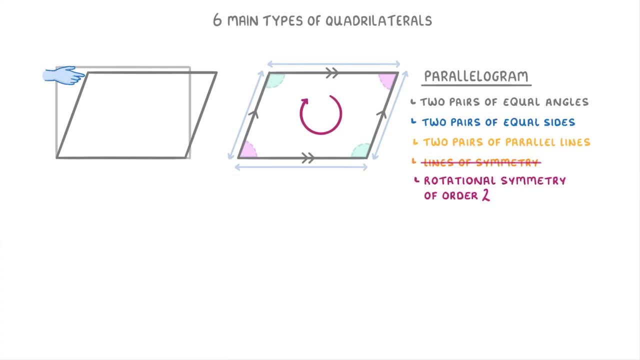 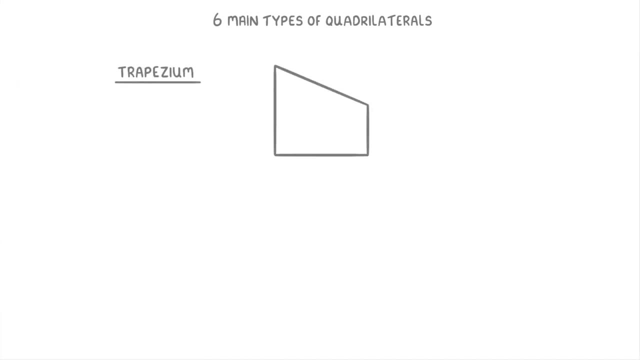 don't have any lines of symmetry, but they do have rotational symmetry of order 2. Now a trapezium is any quadrilateral. that is a full-circuit of a rhombus. Now a trapezium is any quadrilateral. 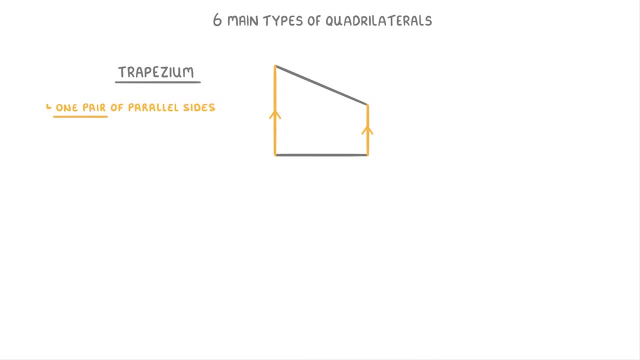 that is a full-circuit of a rhombus, And it's a full-circuit of a rhombus Now, a trapezium is. any only has one pair of parallel sides, and they can often be quite hard to spot. 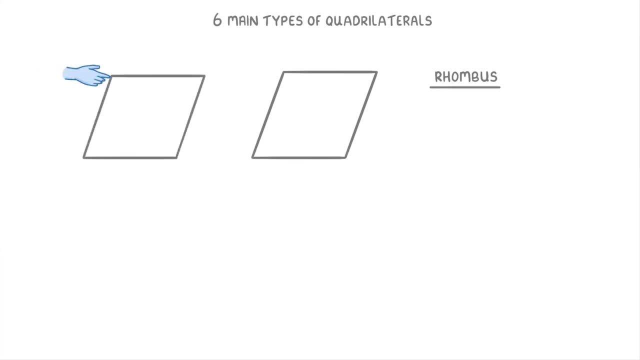 It would sort of lean over to the right. This shape that we're left with is a rhombus. Also, if we rotate it a little bit, then it ends up looking like a diamond. In fact, you might sometimes hear rhombus being called a diamond, but just remember that rhombus. 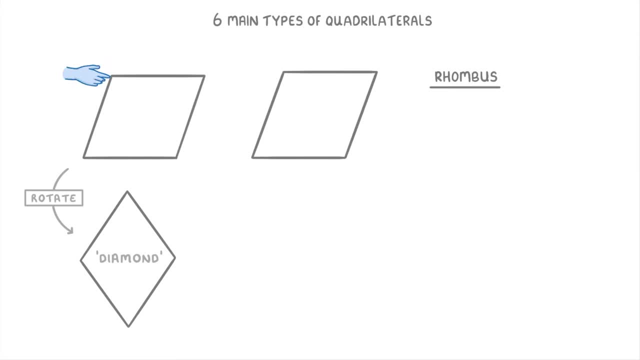 is the proper name for it, Because it came from a square. all four sides of a rhombus are equal length, But because it's been pushed over, the angles aren't 90 degrees anymore. Instead, two of them will be bigger than 90 degrees and equal to each other. 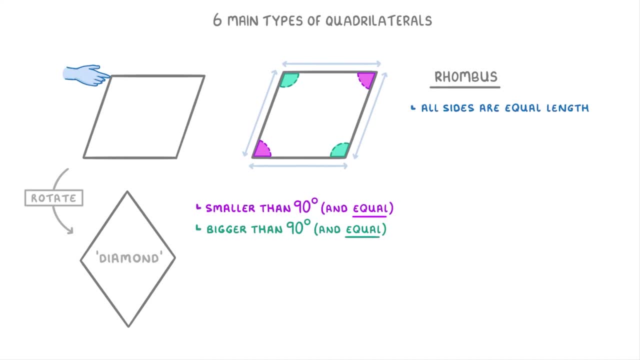 And the other two will be smaller than 90 degrees and equal to each other. So, in total, rhombuses have two pairs of equal angles. They also have two pairs of parallel sides, So these two sides are parallel and these two sides are parallel. 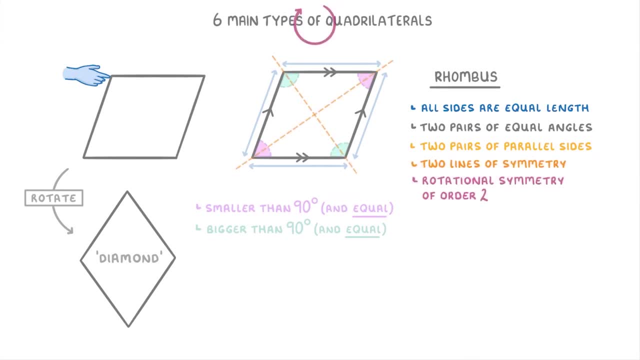 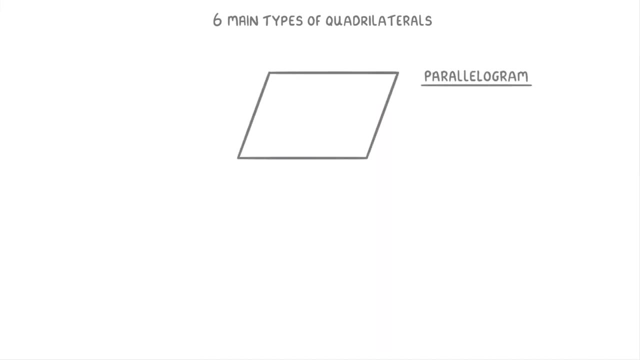 Lastly, they have two lines of symmetry and rotational symmetry of order 2.. Next up, we have the parallelogram, which is very similar to a rhombus, except it's a pushed over rectangle rather than a pushed over square. 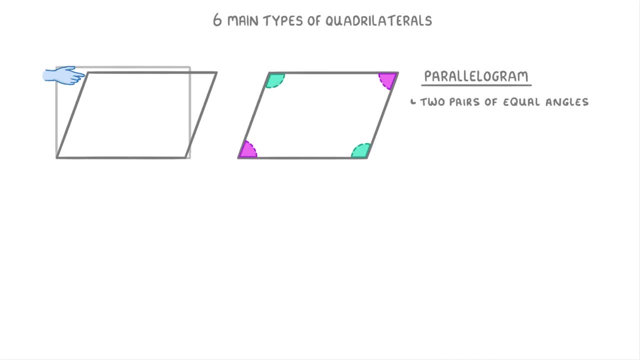 So, just like the rhombus, it has two pairs of equal angles, Because it came from a rectangle, though the sides aren't all the same length. Instead, it has two pairs of equal sides, So these two are equal length and these two are equal length. 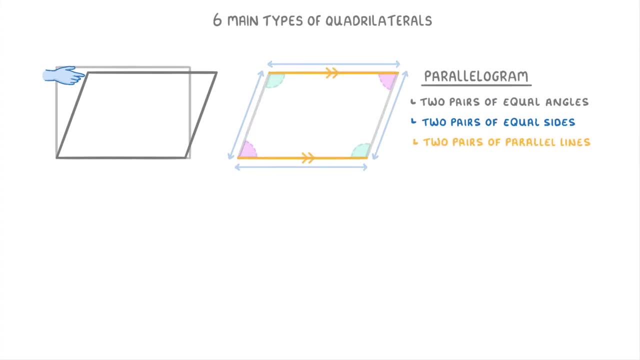 And it also has two pairs of parallel sides. These two and these two Parallelograms don't have any lines of symmetry, but they do have rotational symmetry of order 2. Now, a trapezium is any quadrilateral that only has one. 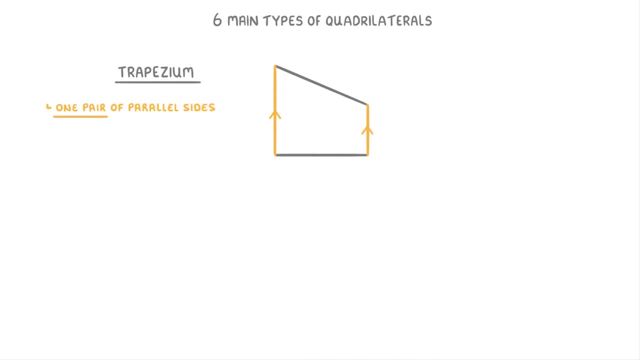 pair of parallel sides, And they can often be quite hard to spot. So if we look at these three shapes as examples, this first one, on the left, would count as a trapezium, because these two sides are parallel, but these two sides aren't.